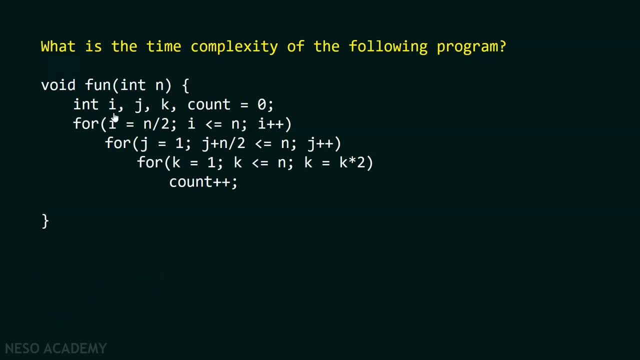 written over here So you can clearly see that the first statement is: I am declaring three variables and one more variable, and I have initialized this variable with value zero. This is a count variable which has been initialized with zero value. Then we have these for loops. 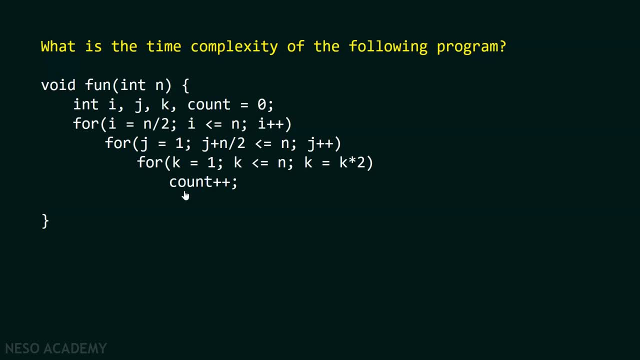 which are basically nested for loops, And within this for loop we have the statement count plus plus. You need to determine the time complexity of this program. It would be better if you can pause the video for a while and try to answer this question on your own. 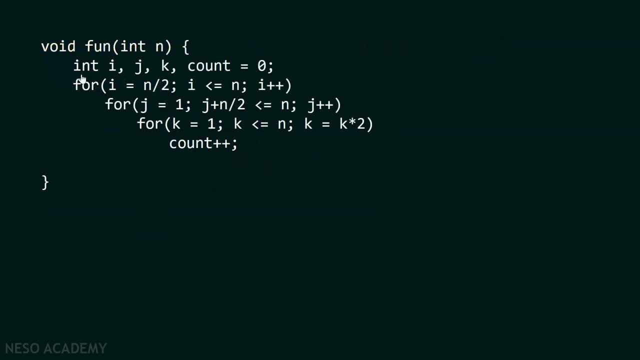 I hope you are done. Okay, let's move on to the solution. Now let's take this statement first. Here you can see I have declared three variables and one more variable, count, which has been initialized to zero. These three variables haven't been initialized. 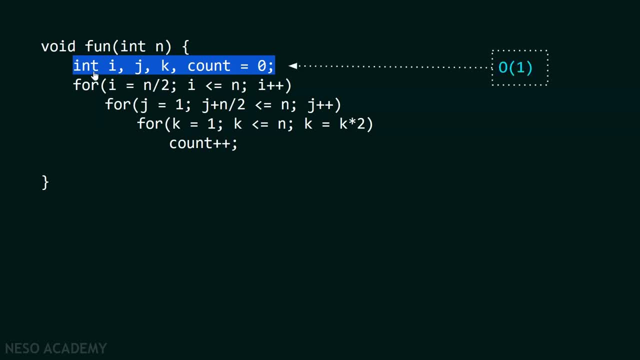 We will use these three variables within this for loops. You can see the time complexity in this case is big of one because it's just taking a constant amount of time for the execution. You know there are no for loops, nothing special, You can treat this. 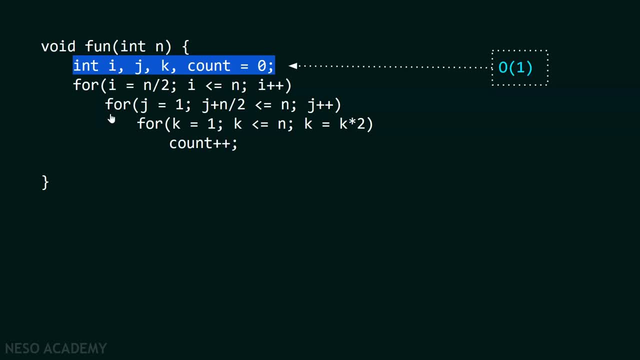 as a single statement, Although you can write these in multiple lines as well, but treat this as a single statement. If you treat them with different statements as well, then also it will take constant amount of time, Isn't that so? So this particular statement. 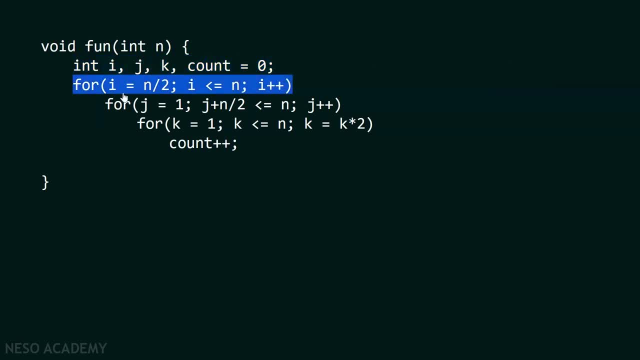 is just taking a constant amount of time. Now let's consider this particular statement. This is nothing but a for loop. right Within this for loop, we have another for loop, And within this for loop, we have another for loop. 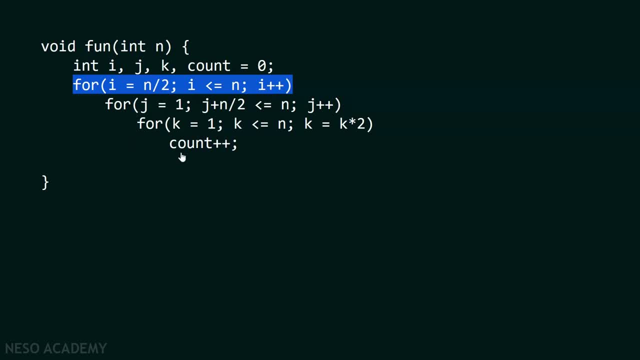 Then we have this statement. Obviously, our task is to find how many times this particular statement has been executed. So let's first evaluate and try to understand what this for loop is and how much time it will take In the iteration number one. 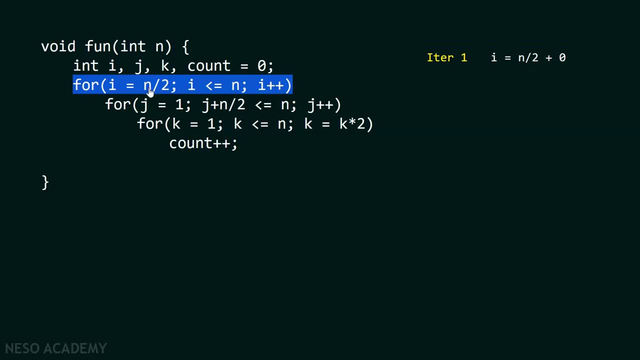 you can clearly see that i is equal to n by two. right, You can write this as: i equals to n by two plus zero. Now in the iteration number one, in the iteration number two, it is clear that this will be: i equals to n divided by two plus one. 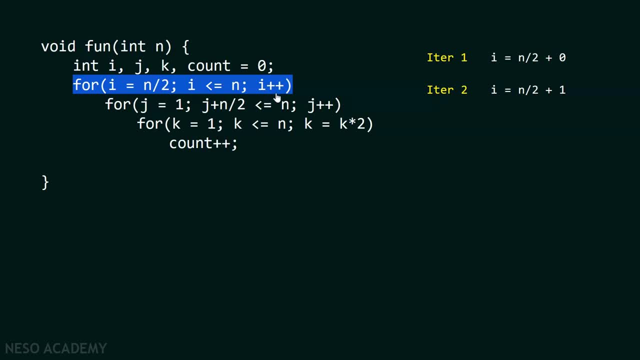 Because you can clearly see over here that this is i plus plus an increment by one step. So obviously in the next iteration this will be n by two plus one. In the iteration number three, this will be n by two plus two. 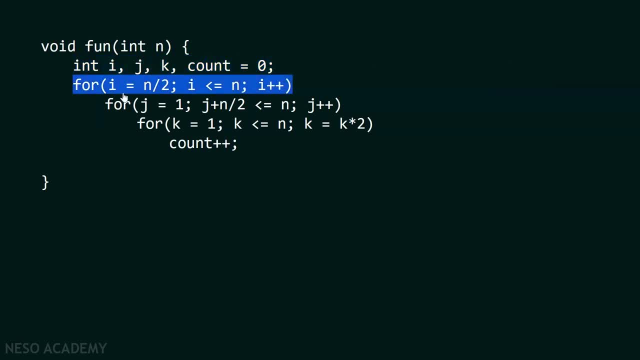 is just taking a constant amount of time. Now let's consider this particular statement. This is nothing but a for loop. right Within this for loop, we have another for loop, And within this for loop, we have another for loop. 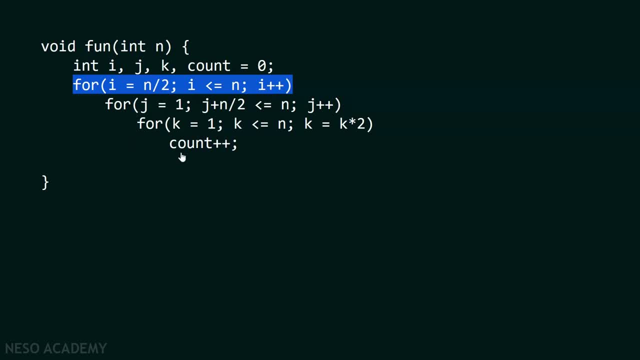 Then we have this statement. Obviously, our task is to find how many times this particular statement has been executed. So let's first evaluate and try to understand what this for loop is and how much time it will take In the iteration number one. 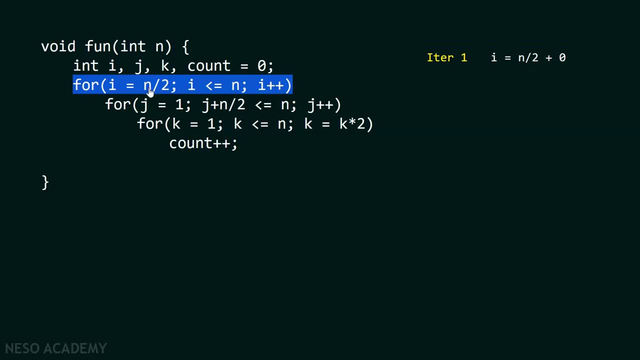 you can clearly see that i is equal to n by two. right, You can write this as: i equals to n by two plus zero. Now in the iteration number one, in the iteration number two, it is clear that this will be: i equals to n divided by two plus one. 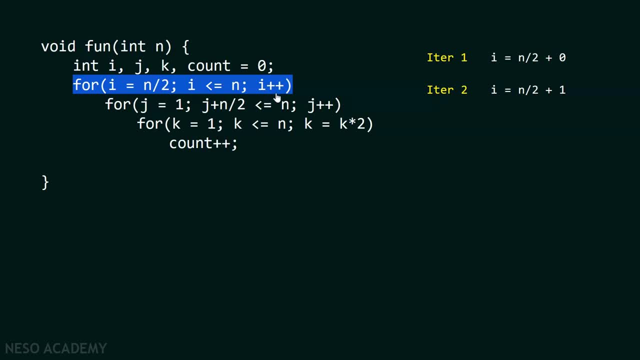 Because you can clearly see over here that this is i plus plus an increment by one step. So obviously in the next iteration this will be n by two plus one. In the iteration number three, this will be n by two plus two. 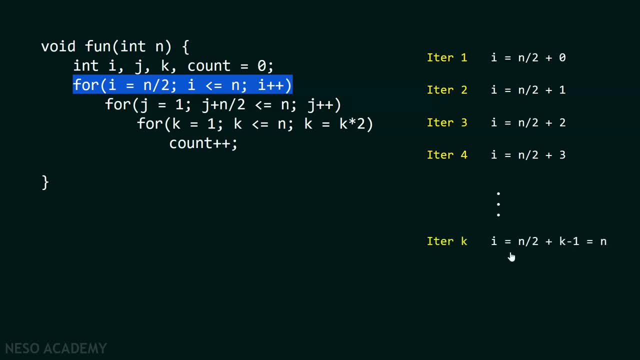 In the iteration number four. this will be n by two plus three, and so on. Now let us assume that we are running up to iteration number k. In that case i will be equal to n by two plus one. Now in the iteration number three. 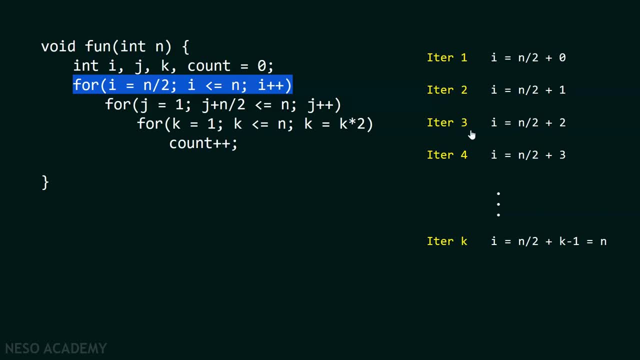 the value is zero. In the iteration number two, this value is one, While this n by two remains constant. only this value is changing with the iterations right. In the iteration number three, this will be two. In the iteration number four, 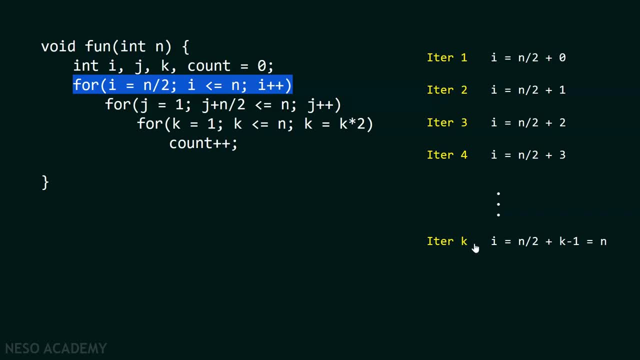 this is three. So similarly, in the iteration number k as well, this will be k minus one. So i will be n by two plus k minus one, which is equal to n. Now let me rewrite this over here in a proper manner. 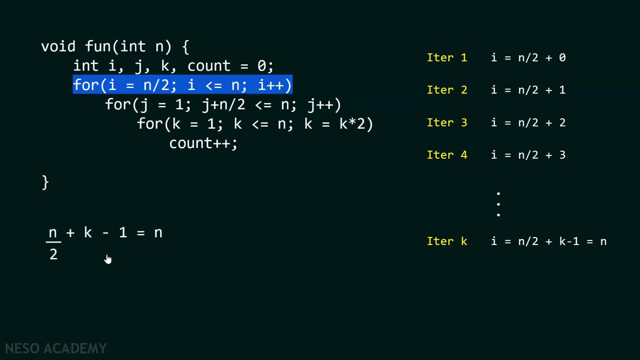 This is n by two plus k minus one, equal to n. Let's solve this. We can write this: k minus one equals to n minus n by two without any problem. I can bring this n by two over here. By solving this, this becomes k minus one. 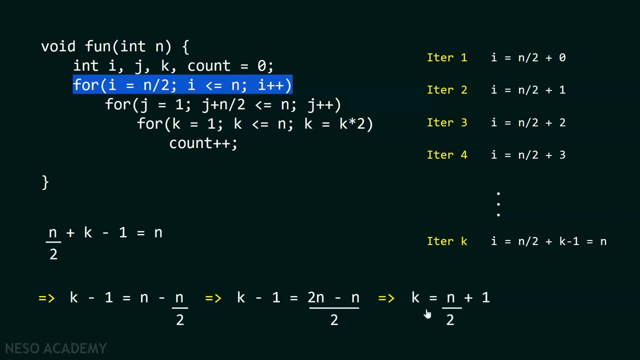 equal to two n minus n divided by two. Again we can write this as: k equals to n by two plus one. This means that our loop is running n by two times. I can take the least upper bound as n without any problem. 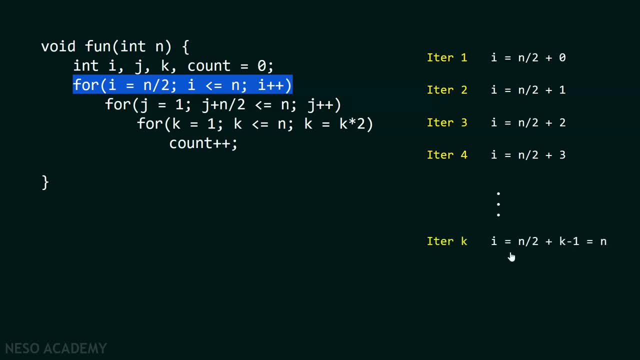 In the iteration number four. this will be n by two plus three, and so on. Now let us assume that we are running up to iteration number k. In that case i will be equal to n by two plus k minus one. So i will be n by two plus k minus one. 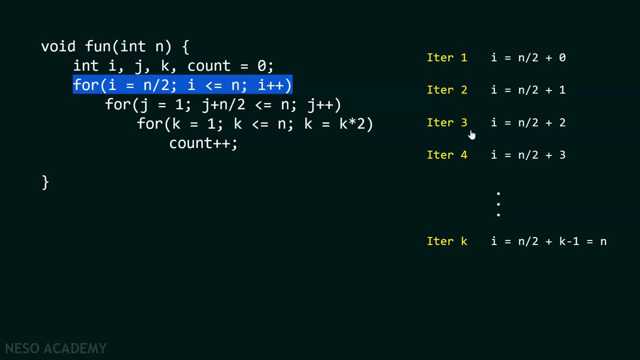 i equals to n, Because this is the last iteration we are considering, But we do not know how many times this has been executed. That is why I have taken this as k. So at this particular iteration, i is equal to n by two plus k minus one. 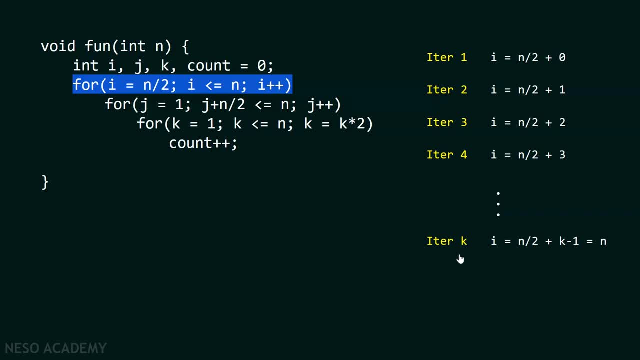 which is equal to n- Because this is the last iteration we are considering, But we do not know how many times this has been executed- which is equal to n. Now let me rewrite this over here in a proper manner. This is n by two plus k minus one, equal to n. 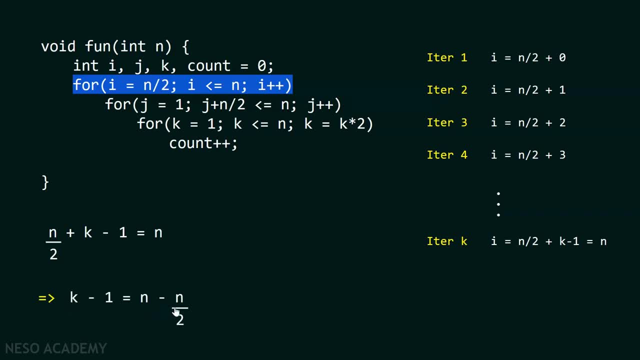 Let's solve this. We can write this: k minus one equals to n minus n by two without any problem. I can bring this n by two over here. By solving this, this becomes k minus one equal to two, n minus n divided by two. 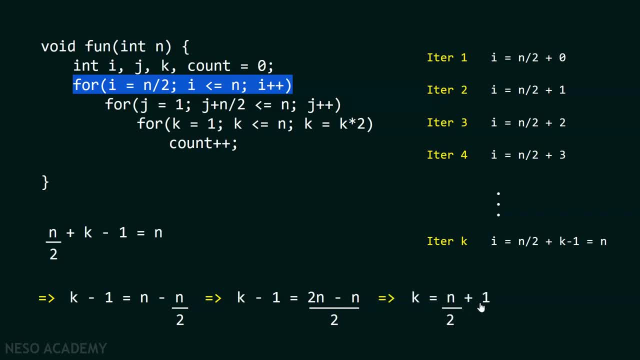 Again we can write this as: k equals to n by two plus one. This means that our loop is running n by two times. I can take the least upper bound as n without any problem. Loop executes n by two plus one, which can be thought of as n by two. 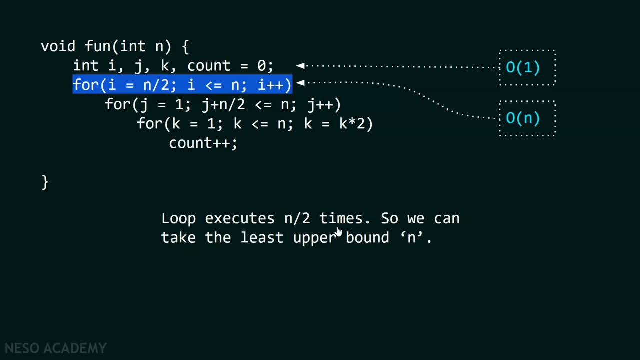 times only because plus one. if we won't consider then it will not cause any problem. We can take the least upper bound as n without any problem. So this loop is actually running n times, Although it is running n by two times. 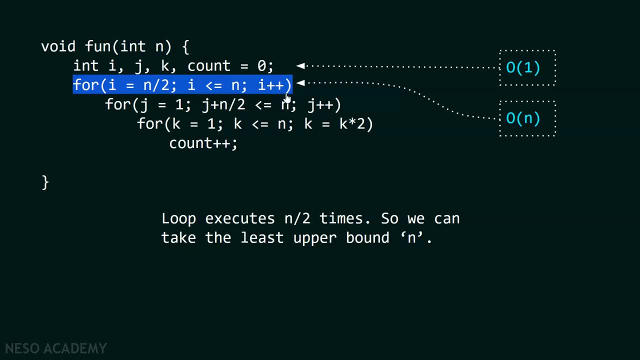 let me tell you. but we are taking the least upper bound without considering the constants. So least upper bound of n by two is obviously n, So we can say that this loop is running n times. So this is big O of n. 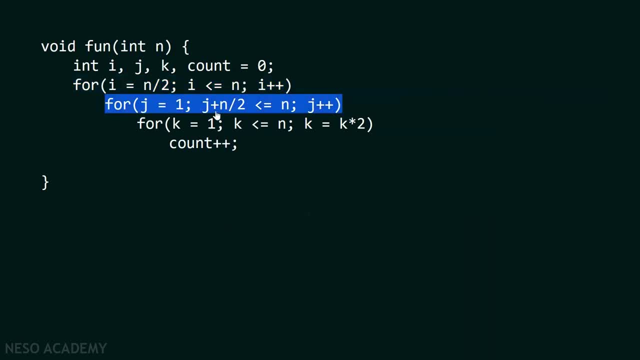 Now let's consider the next loop Here. in this case, you have j equals to one, and this is quite interesting. Here it is written j plus n, divided by two less than or equal to n, And here it is just j plus plus. 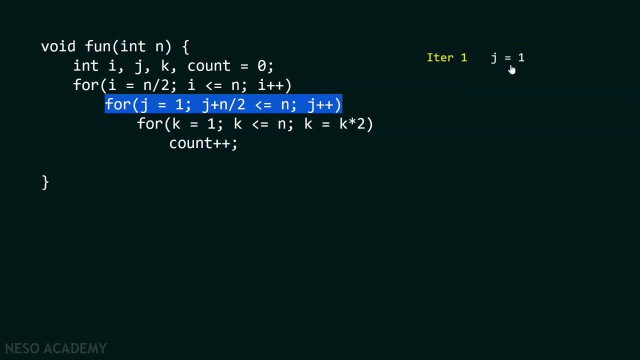 Let's see what is happening over here. In the iteration number one, it is clear that j is equal to one right. In the iteration number two, j is equal to two. Iteration number three: j is equal to three. Iteration number four: j is four, and so on. 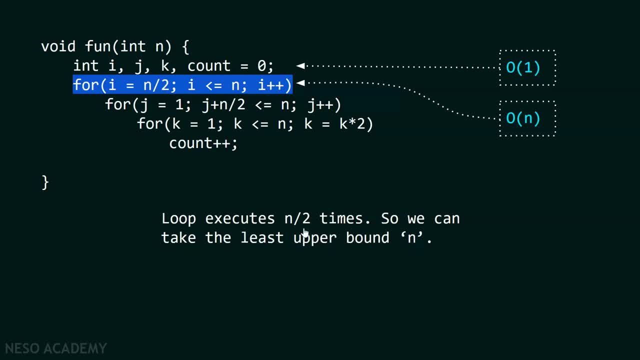 Loop executes n by two plus one, which can be thought of as n by two times only because plus one- if we won't consider then it will not cause any problem. We can take the least upper bound as n without any problem. So this loop is actually running n times. 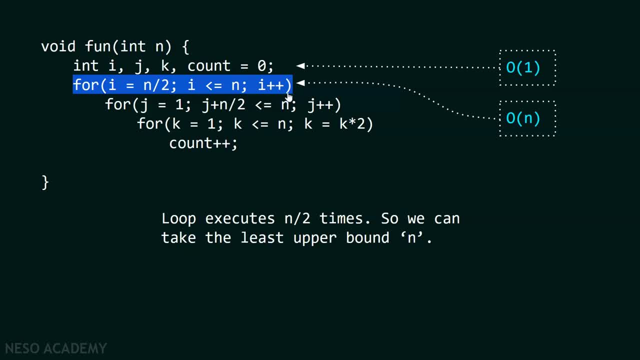 Although it is running n by two times, let me tell you. but we are taking the least upper bound without considering the constants. So least upper bound of n by two is obviously n, So we can say that this loop is running n times. 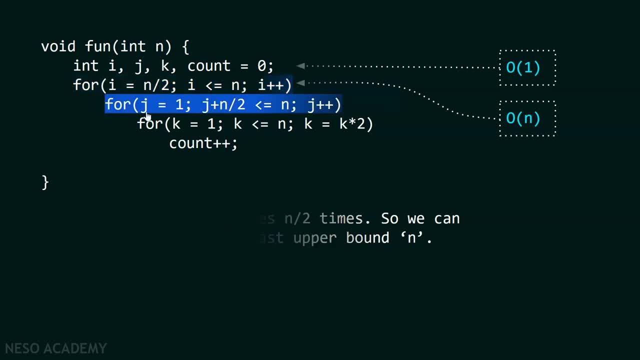 So this is big O of n. Now let's consider the next loop. Here, in this case you have j equals to one, and this is quite interesting. Here it is written j plus n divided by two less than or equal to n. 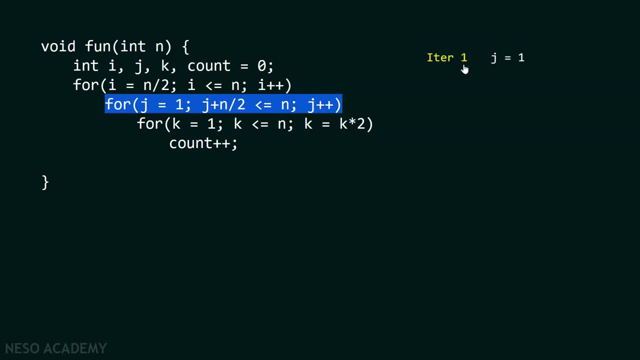 And here it is just j plus plus. Let's see what is happening over here. In the iteration number one, it is clear that j is equal to one right. In the iteration number two, j is equal to two. Iteration number three: j is equal to three. 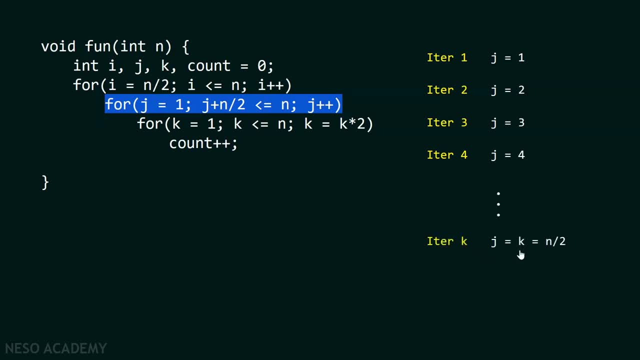 Iteration number four: j is four, and so on. At iteration number k, j will be equal to k, without any problem, because here in iteration number four, we have j equals to four. Iteration number three: we have j equals to three. 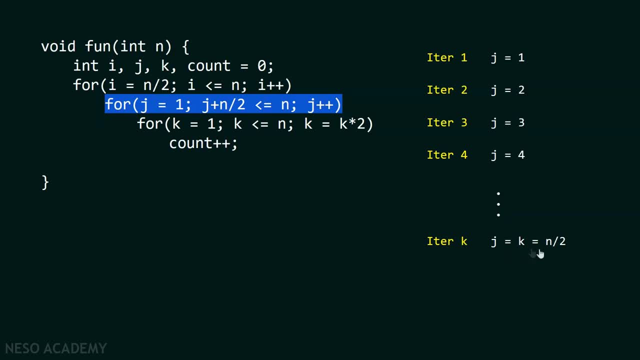 So it is clear that in iteration number k, j is equal to k, which is equal to n by two, Why I am writing this as n by two. j plus n by two less than or equal to n can be written as j, less than or equal to. 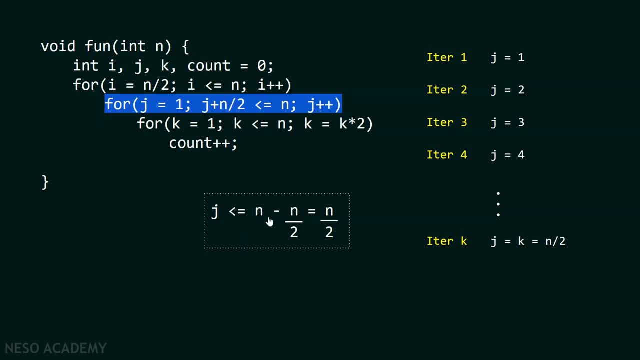 n minus n by two. I can bring this n by two over here. This becomes n minus n by two. I can solve this and this brings me n by two. So j is eventually less than or equal to n by two. I can say that k is equal to. 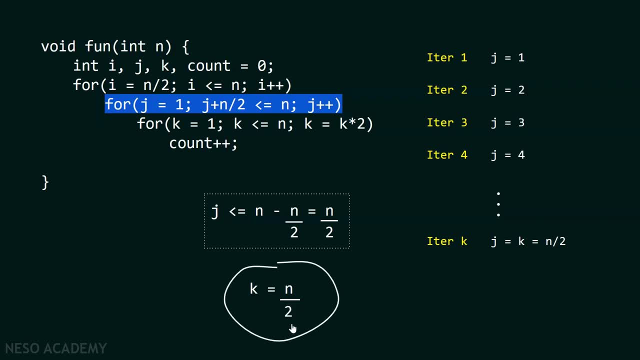 n by two without any problem. So it is clear from this fact that this loop is running n by two times. I can take the upper bound as n by two and can clearly say that loop is running with the time complexity O. So this is the upper bound I can take. 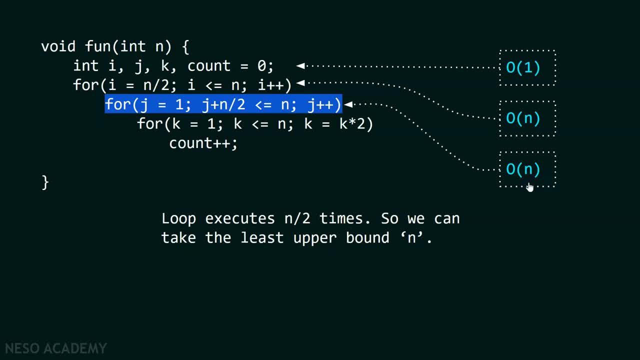 which is n instead of n by two. Always try to remove the constants. Don't take n by two. Instead of n by two, you can take a least upper bound. That could be n. Now let's see the other loop. 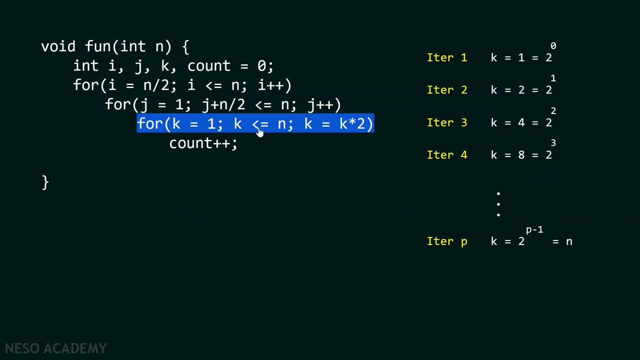 Here. in this case, obviously we can clearly understand that k is equal to one and k is less than or equal to n and k is equal to k into two. We have already calculated the time complexity when these loops are available In iteration number one. k is equal to one. 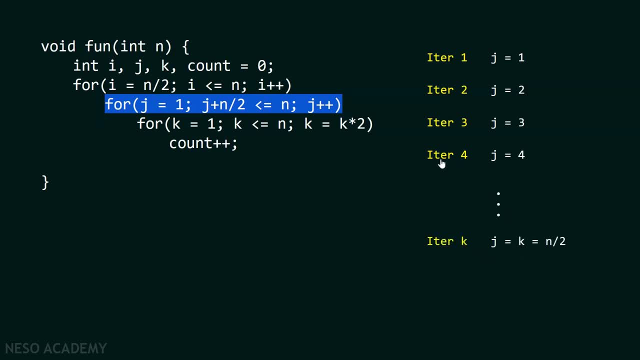 At iteration number k, j will be equal to k without any problem, because here in iteration number four, we have j equals to four. Iteration number three: we have j equals to three. So it is clear that in iteration number k 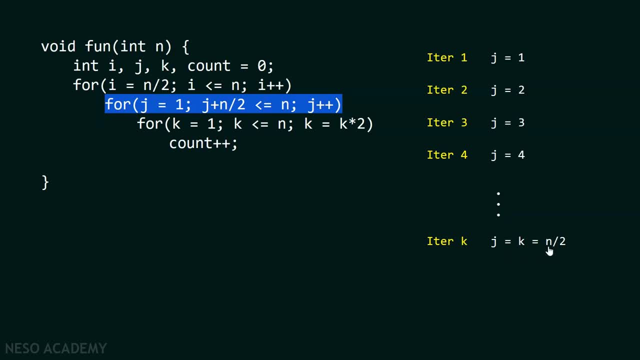 j is equal to k, which is equal to n by two, Why I am writing this as n by two. j plus n by two. less than or equal to n can be written as j less than or equal to n minus n by two. I can bring this n by two over here. 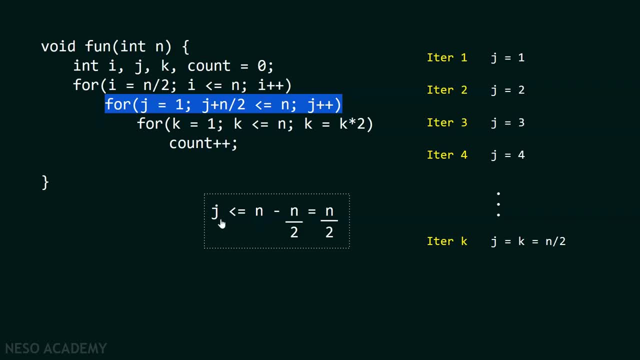 This becomes n minus n by two. I can solve this and this brings me n by two. So j is eventually less than or equal to n by two. I can say that k is equal to n by two without any problem. So it is clear from this fact that 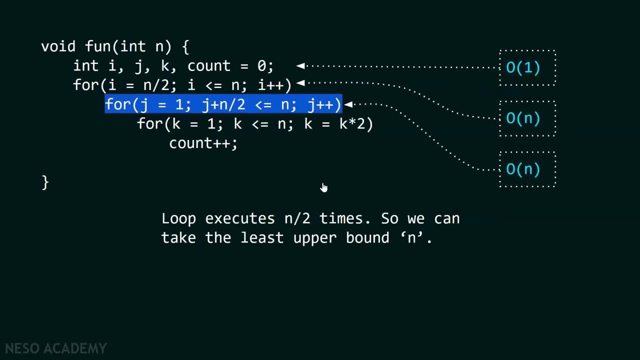 this loop is running n by two times. I can take the upper bound as n by two and can clearly say that loop is running with the time complexity O. So this is the upper bound I can take, which is n instead of n by two. 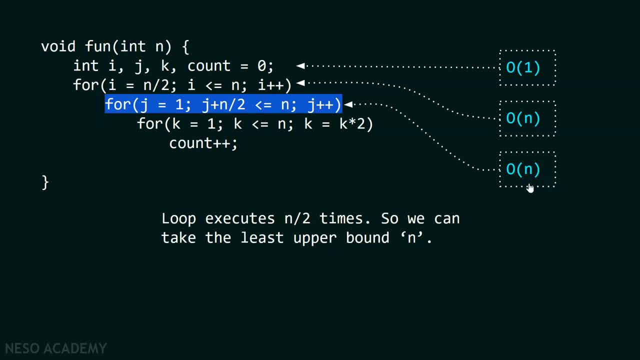 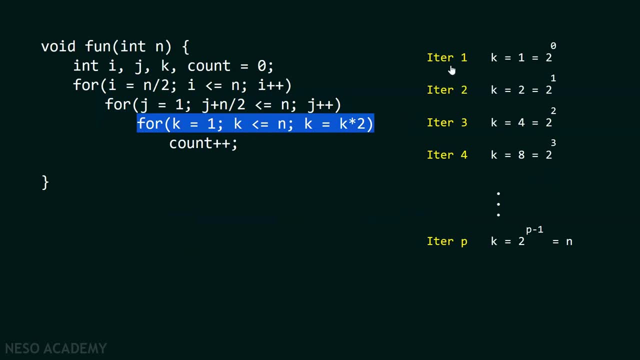 Always try to remove the constants. Don't take n by two. Instead of n by two, you can take a least upper bound. That could be n. Now let's see the other loop Here. in this case, obviously, we can clearly understand that k is equal to one. 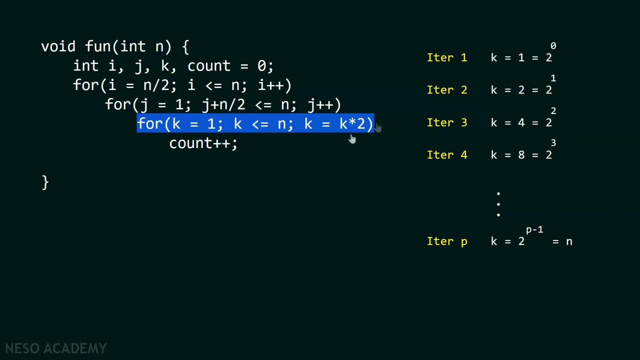 and k is less than or equal to n and k is equal to k into two. We have already calculated the time complexity when these loops are available In iteration number one. k is equal to one. One can be written as two to the power zero. 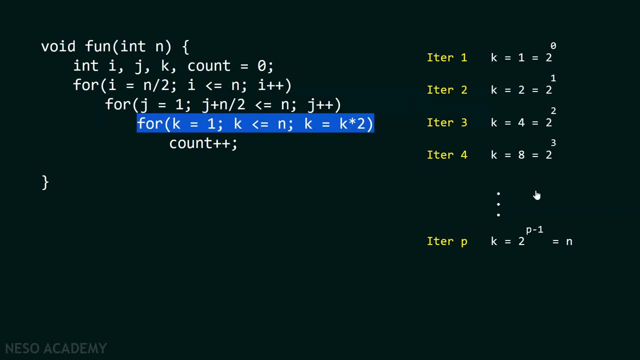 Two can be written as two to the power one. Similarly, eight can be written as two to the power three, and so on. If I consider this up to iteration number p, then this will be two to the power p minus one, which is eventually equal to n. 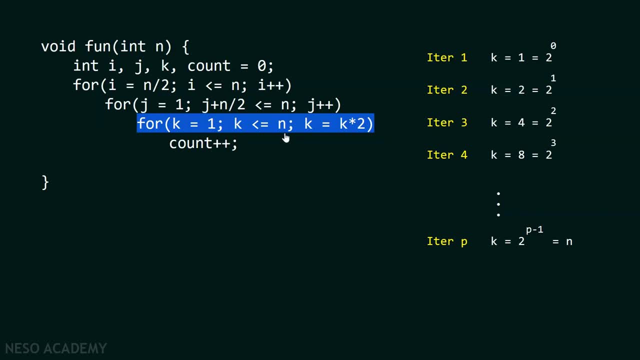 Because in the last iteration two to the power p minus one is equal to n. You can clearly see over here I can say that two to the power p minus one is equal to n, or n is equal to two to the power p minus one. 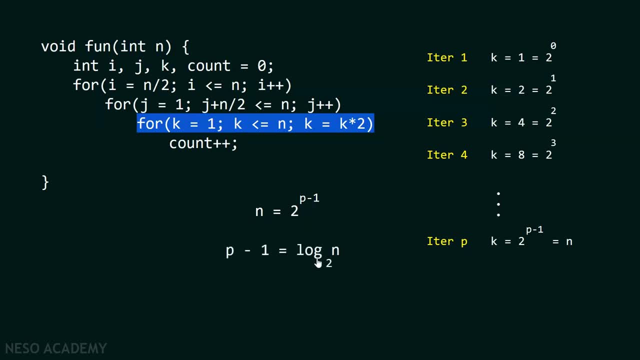 without any problem. I can take log on both sides. I can write this as: p equals to log n, base two plus one, which is equal to big O of log n. I can eliminate this constant, So I can say that the time complexity for this loop. 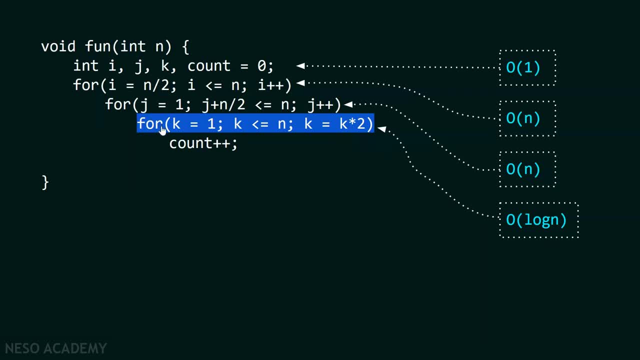 is big O of log n. Now let me tell you these are nested for loops, So obviously you know that we need to multiply these three time complexities, n into n, into log n, which is equal to big O of n square log n. 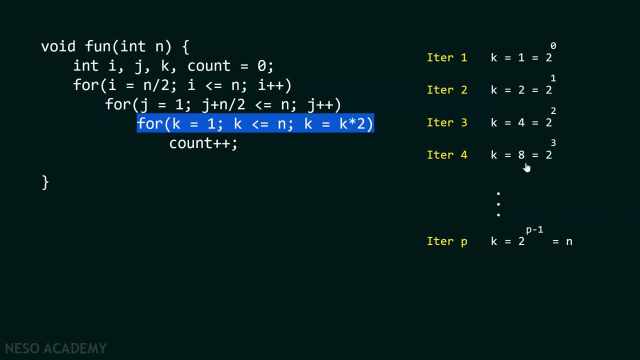 One can be written as two to the power zero. Two can be written as two to the power one. Similarly, eight can be written as two to the power three, and so on. If I consider this up to iteration number p, then this will be two to the power p minus one. 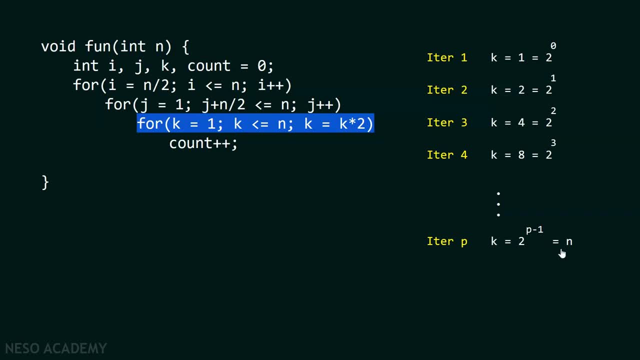 which is eventually equal to n, Because in the last iteration two to the power p minus one is equal to n. You can clearly see over here I can say that two to the power p minus one is equal to n, or n is equal to two to the power p minus one. 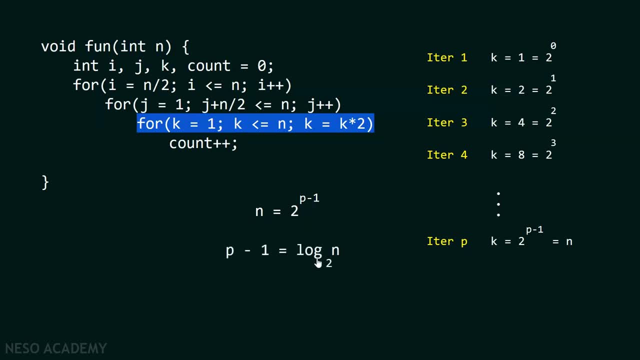 without any problem. I can take log on both sides. I can write this as: p equals to log n, base two plus one, which is equal to big O of log n. I can eliminate this constant, So I can say that the time complexity for this loop. 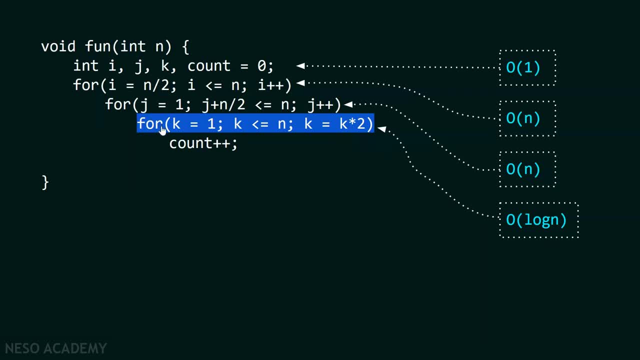 is big O of log n. Now let me tell you these are nested for loops, So obviously you know that we need to multiply these three time complexities, n into n, into log n, which is equal to big O of n square log n. 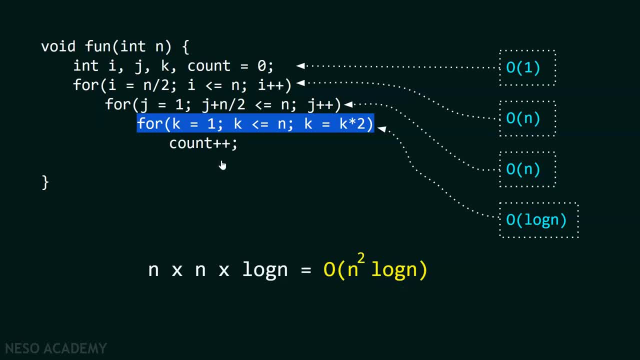 So I can say that the time complexity for this particular code is big O of n square log n, or order of n square log n. So this is the time complexity of this particular code. This loop is running n times. I have taken the upper bound. 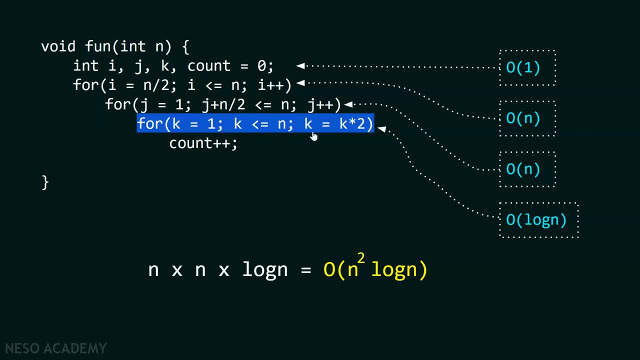 This loop is also running n times. Again, I have taken the upper bound Here. in this case, this loop runs log n times. This is nested for loop structure. So here, in this case, we need to multiply these three time complexities. 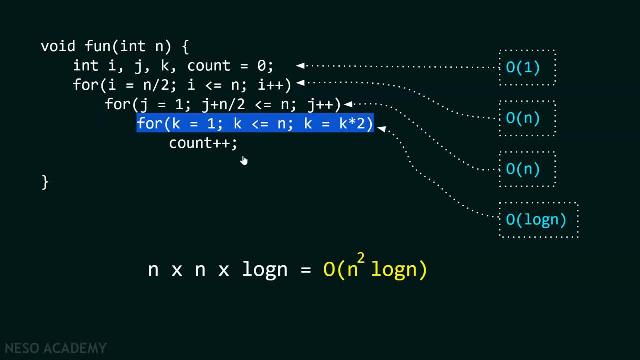 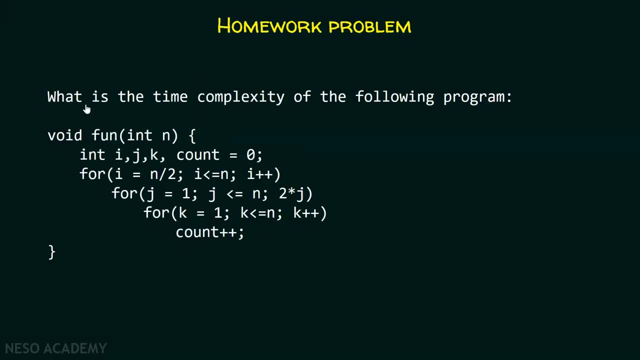 n into n into log n will give us n square log n, which is the final time complexity. This statement is executing n square log n times, So this is the time complexity of this particular code. Now here is one homework problem for you. 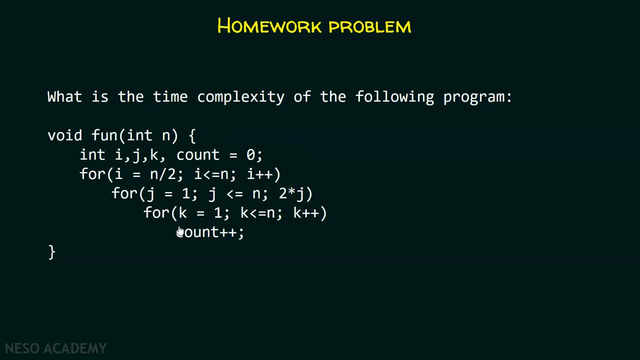 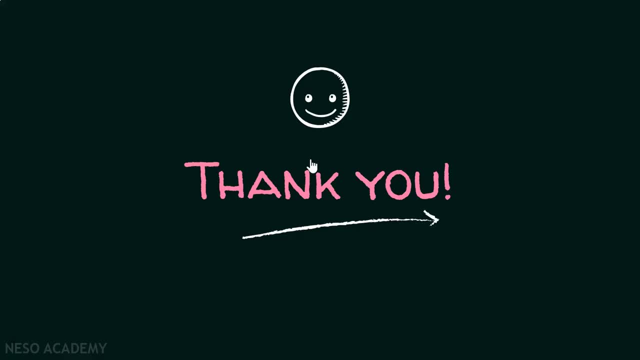 The program is available in front of you. Again, we have three nested for loops. You need to determine the time complexity of this program And obviously you can post your answers in the comment section below. Okay, friends, this is it for now. Thank you for watching this presentation. 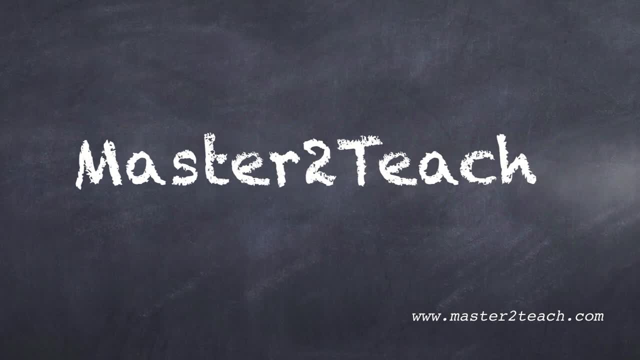 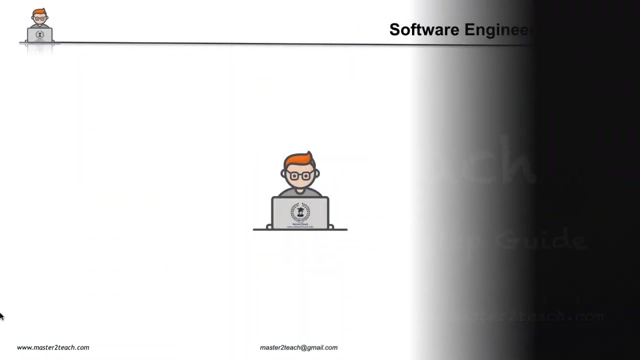 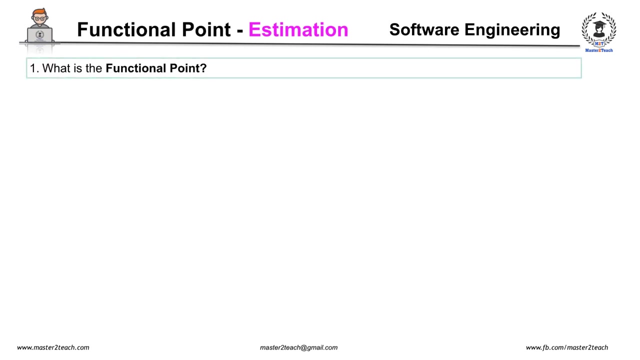 Hello everyone, welcome to master2teach step-by-step guide. In this video you will learn what is functional point in software engineering, how to calculate functional point for project estimation, and we will see the examples of functional point calculation with its uses.